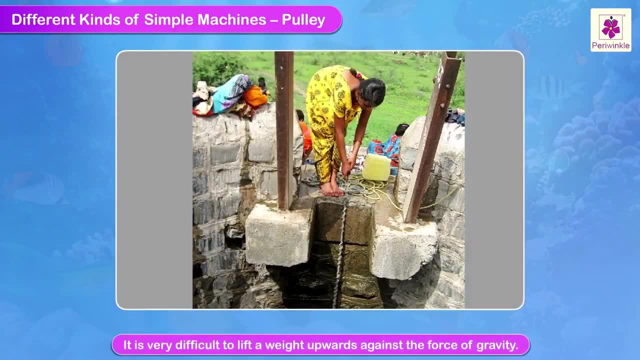 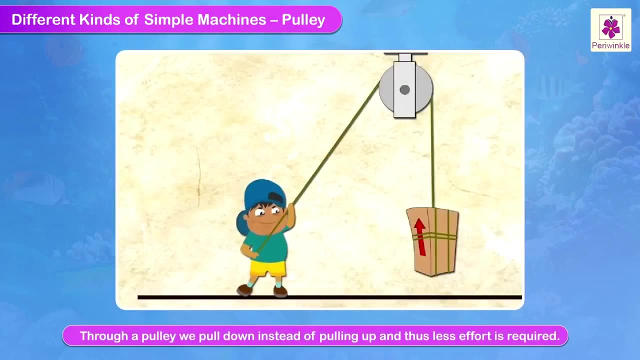 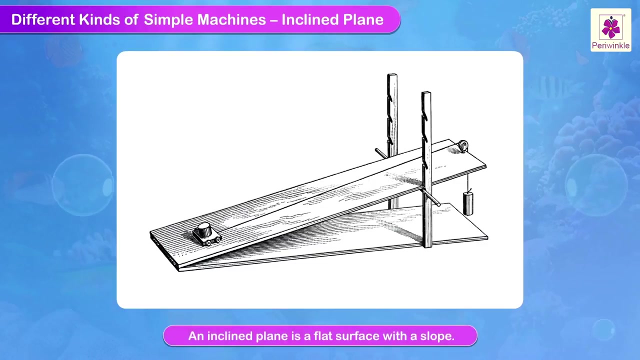 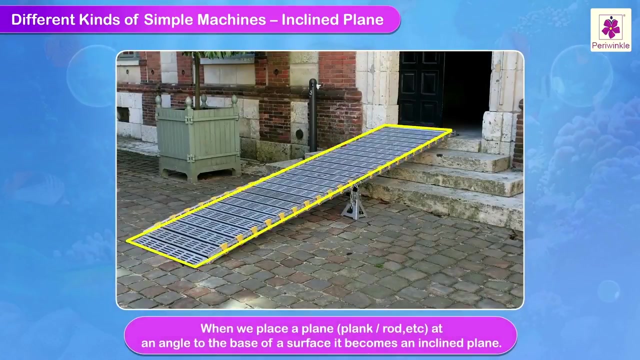 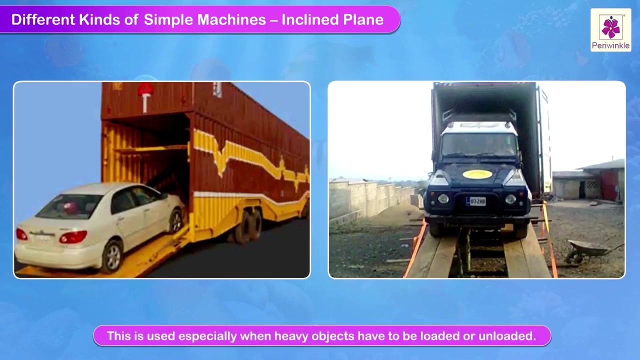 It is very difficult to lift a weight upwards against the force of gravity, But through a pulley we pull down instead of pulling up, and thus less effort is required. Simple Machines, The Justice of rope. The truth is that the Federal bank of India is one of the largest. 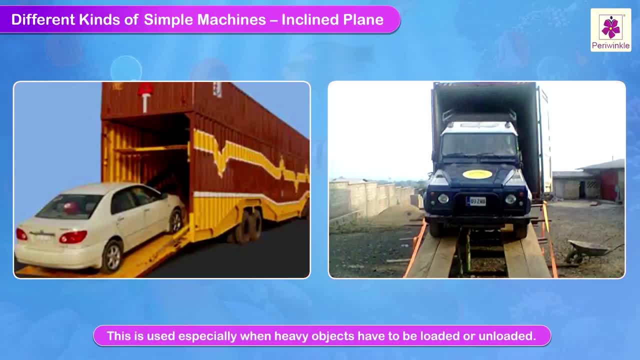 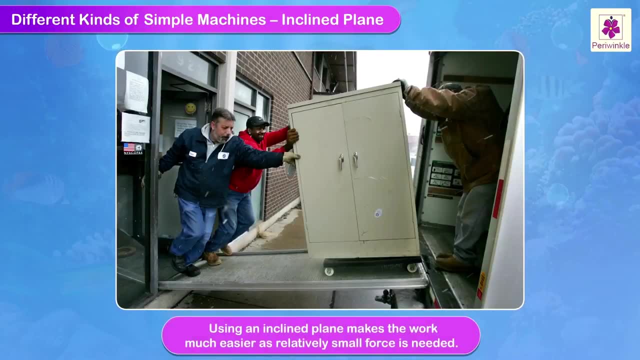 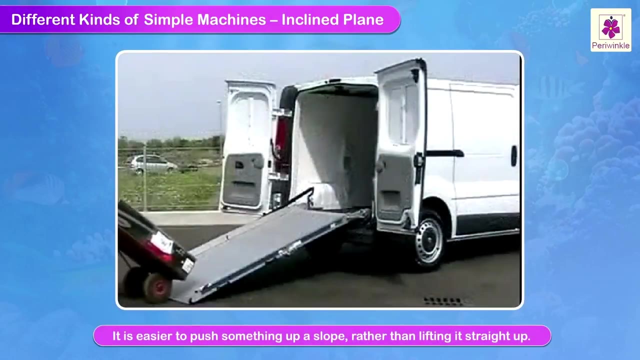 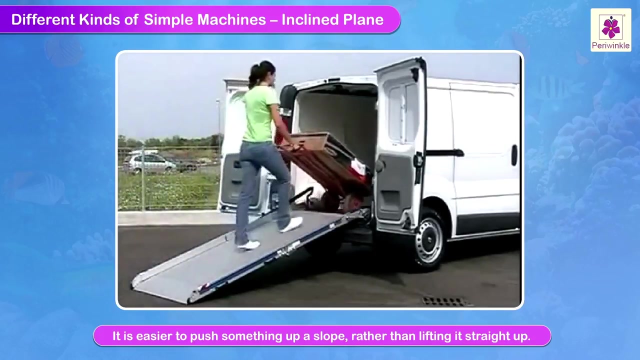 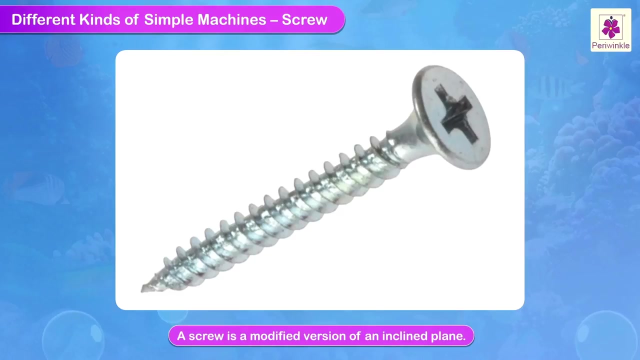 and best spinning academia for or unloaded. Using an inclined plane makes the work much easier, as relatively small force is needed. It is easier to push something up a slope rather than lifting it straight up A screw. A screw is a modified version of an inclined plane. It is actually an inclined. 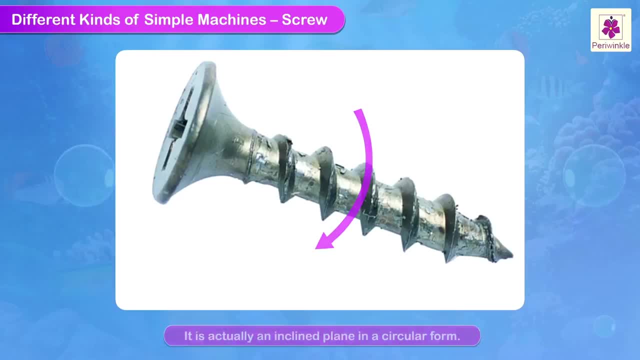 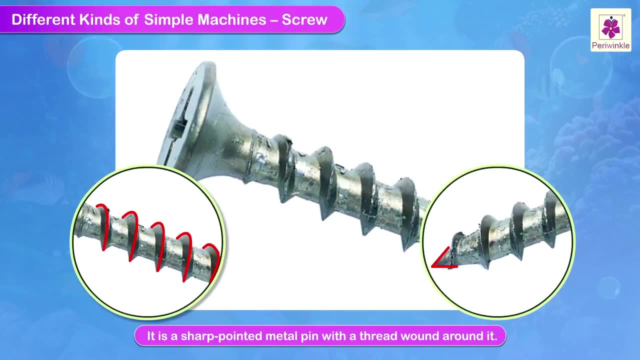 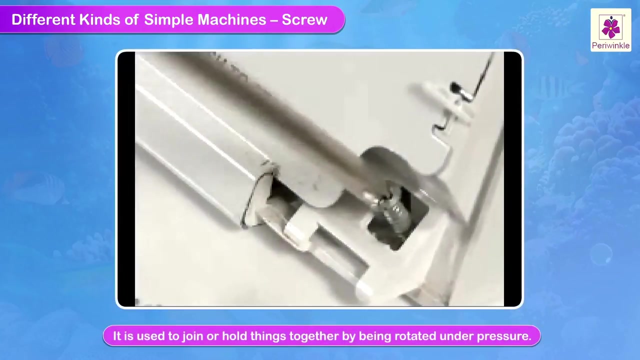 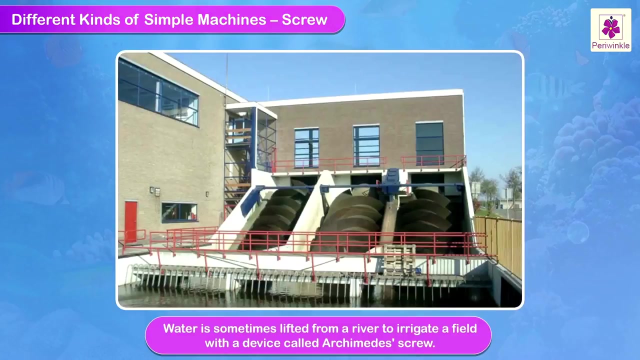 plane in a circular form. It is a sharp pointed metal pin with a thread wound around it. It has a slotted head. It is used to join or hold things together by being rotated under pressure. Water is sometimes lifted from a river to irrigate a field with a device called Archimedes screw. 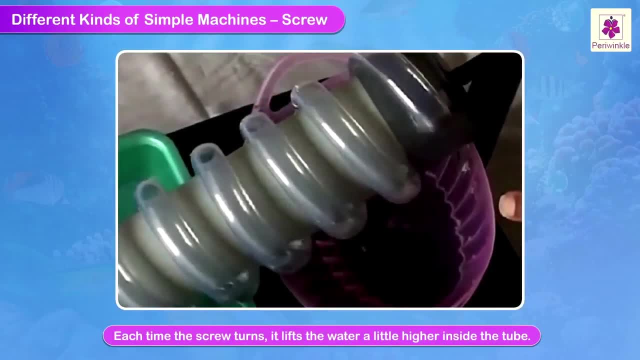 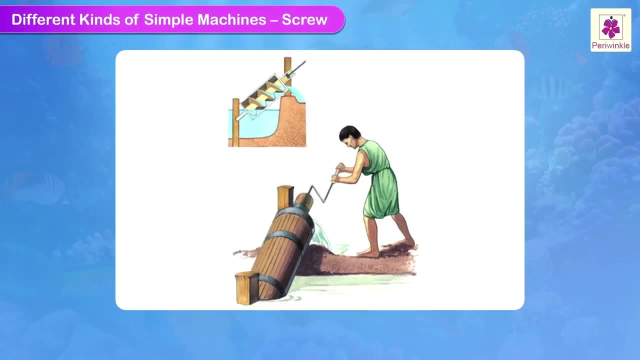 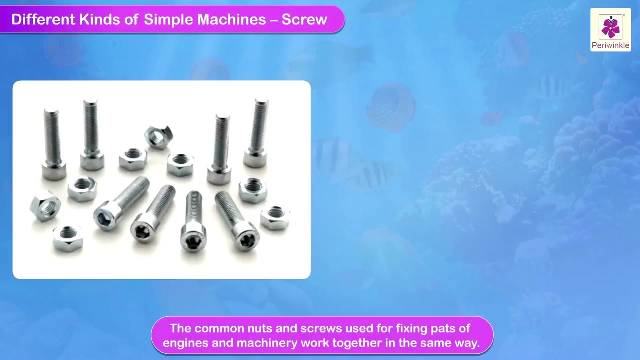 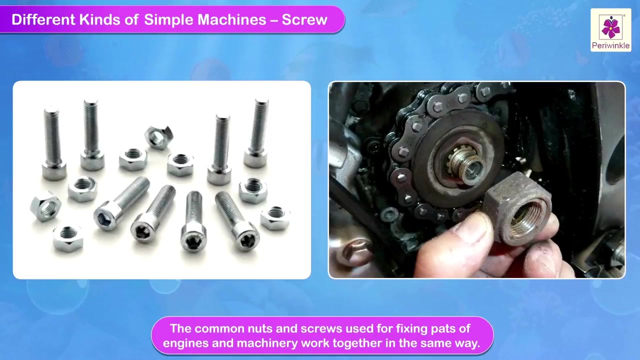 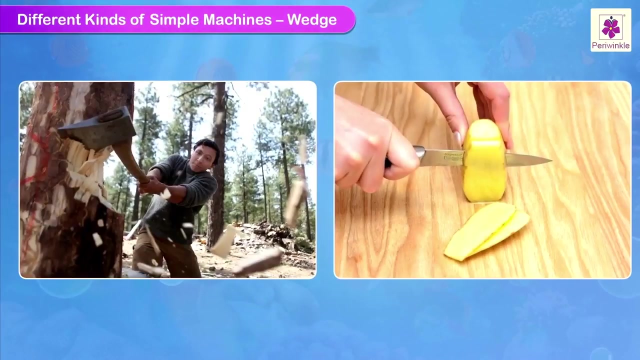 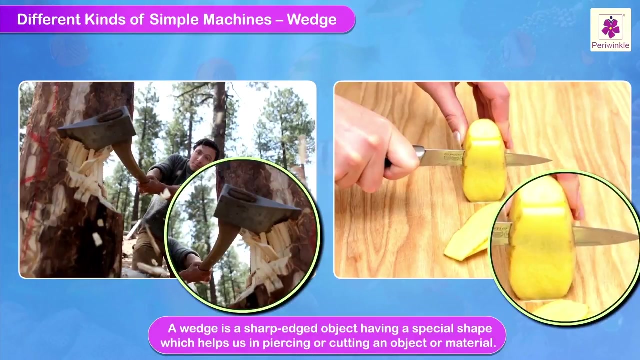 Each time the screw turns it lifts water a little bit higher up inside a tube. It was a commonly used device in Egypt. The common nuts and screws used for fixing parts of engines and machinery work together in the same way. Simple machines Wedge. A wedge is a sharp edged object having a special shape which helps us in piercing. 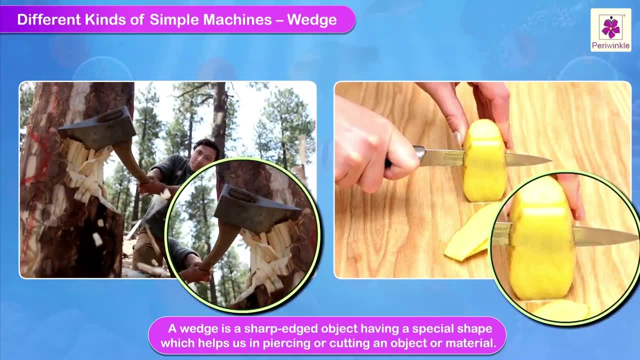 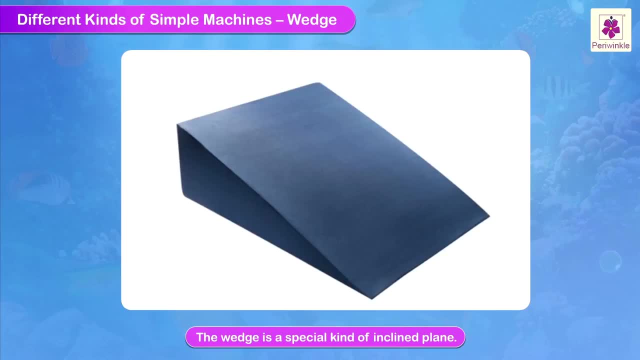 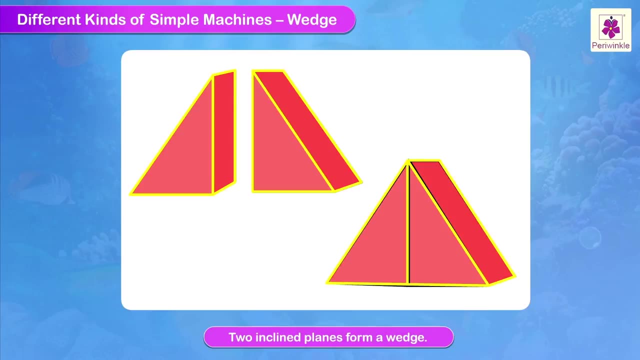 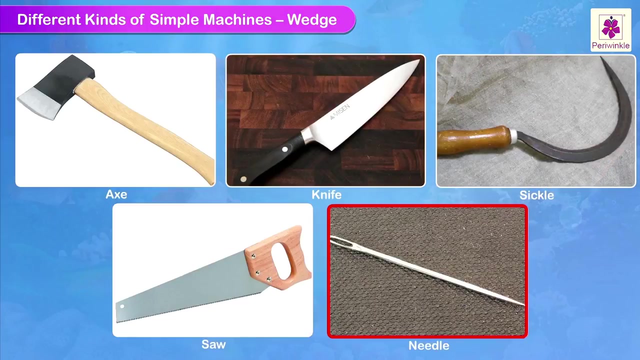 cutting or cutting an object or material. The wedge is a special kind of inclined plane. Place two inclined planes back to back and we get a wedge. Axe, Knife, Sickle, Saw, Needle are examples of wedge. For more information on wedge maintenance, please visit our website. 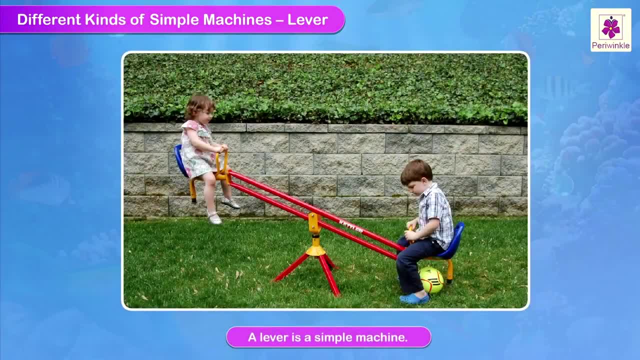 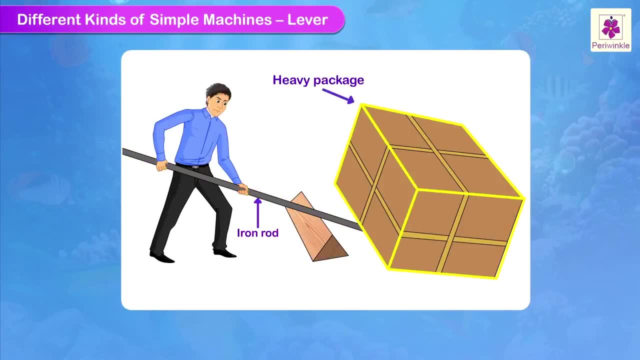 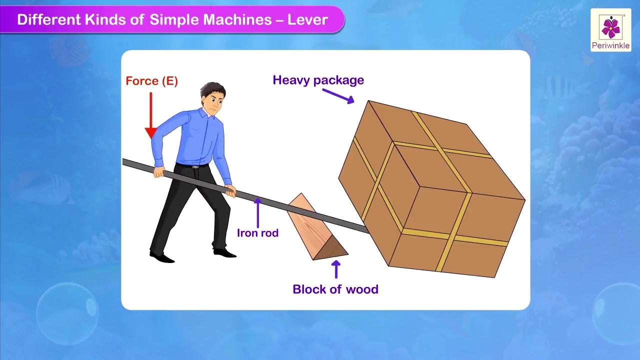 Liver. A liver is a simple machine. The man is using an iron rod to lift the heavy package. He has placed a block of wood close to the package and he is resting the rod on it. He applies a downward force and thus is able to lift the package. 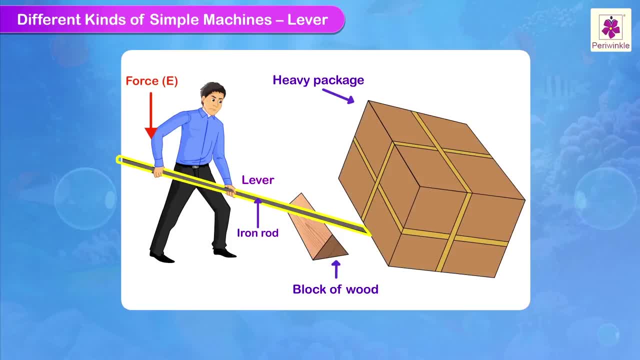 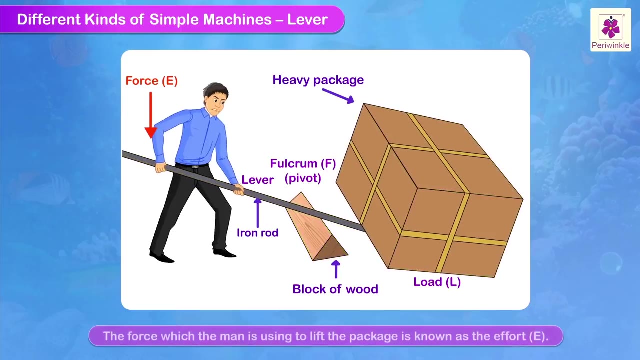 Here, the iron rod is the liver. The package to be lifted is the load. The wooden block is the fulcrum, also called a pivot, which is the fixed point of the liver. The force which the man is using to lift the package is known as the effort. 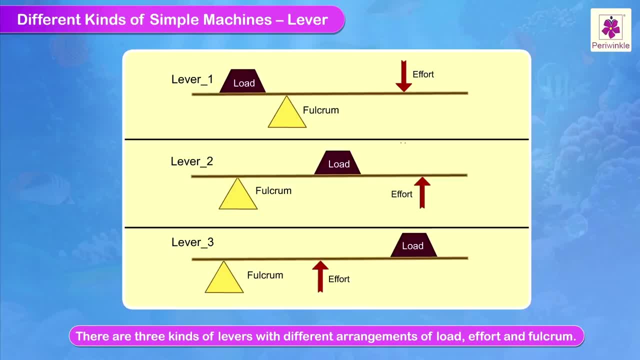 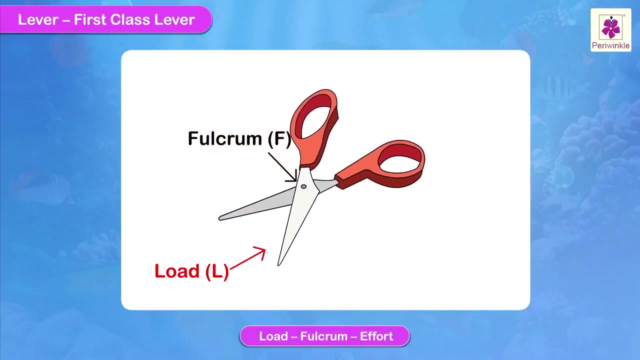 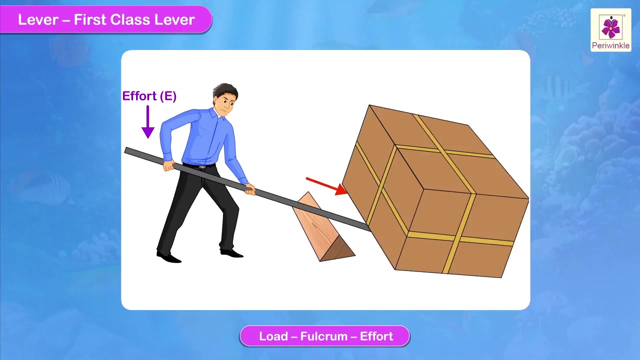 There are three kinds of liver. There are two types of liver which are different arrangements of load, effort and fulcrum. First class liver. Load, fulcrum effort: The effort put at one end of the rod is transferred to the other end of the rod, which is pushed. 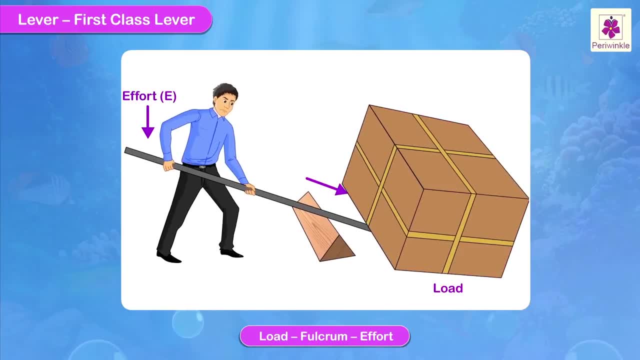 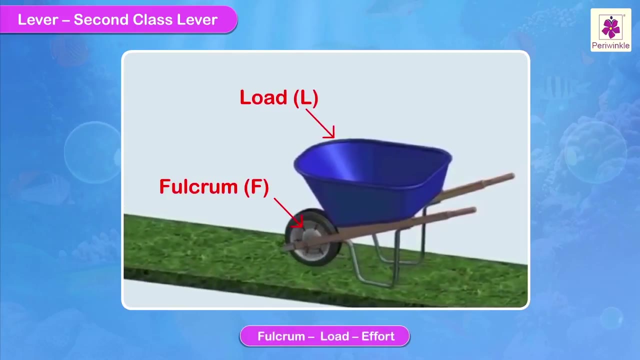 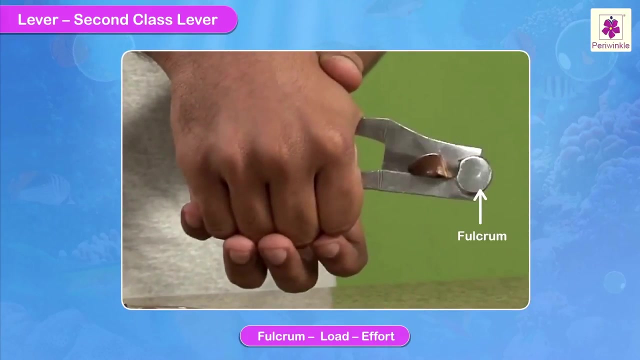 under the load and the work gets done Here, Here, Here, Finally, the fulcrum is between the load and effort. Second class liver Fulcrum, load effort. In these types of livers the fulcrum is at one end, the effort is applied at the other.